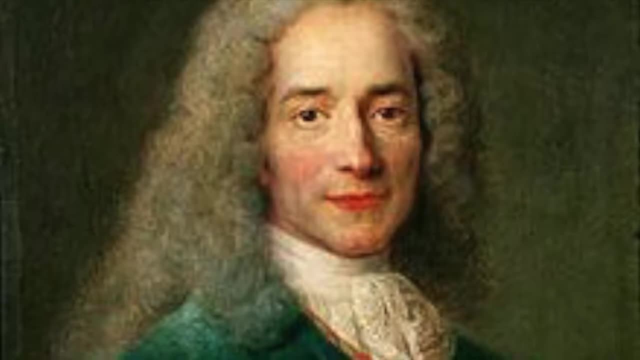 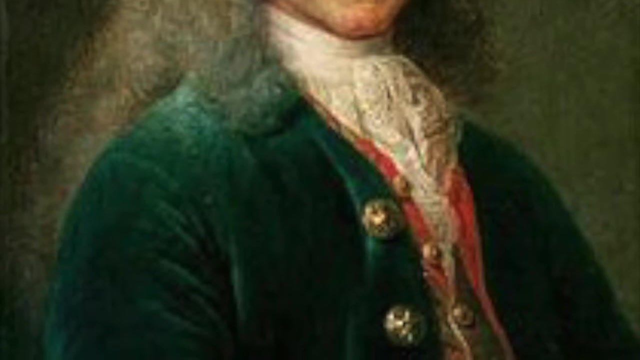 reason for obtaining knowledge, along with empiricism, which stresses the use of sense perception rather than pure reason. Rationalism was one of the main intellectual currents of the Enlightenment, a cultural movement spanning the 17th and 18th centuries that revolutionized the Western world, Along with men like John Locke, John Hobbes and Voltaire, Descartes spurred society to re-examine its traditions and institutions, leading to major societal upheaval. Both the American and French revolutions were based on Enlightenment theories, in part from Descartes and the way we approach science. 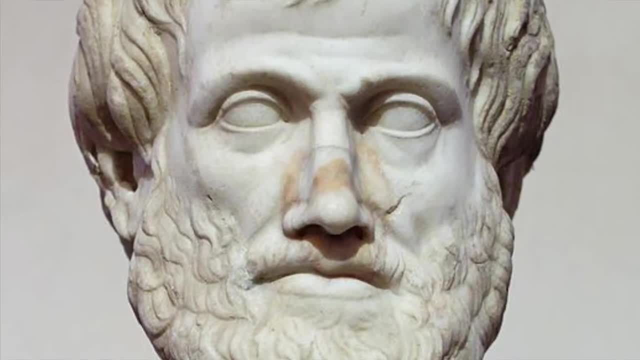 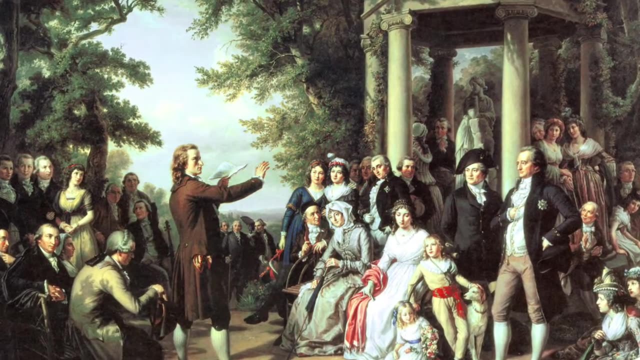 math, philosophy and the idea of self were radically transformed. during this period, Descartes was both influenced and influenced many important philosophers. His most notable influences were Plato, Aristotle and theologians of the 19th century. Descartes was a great 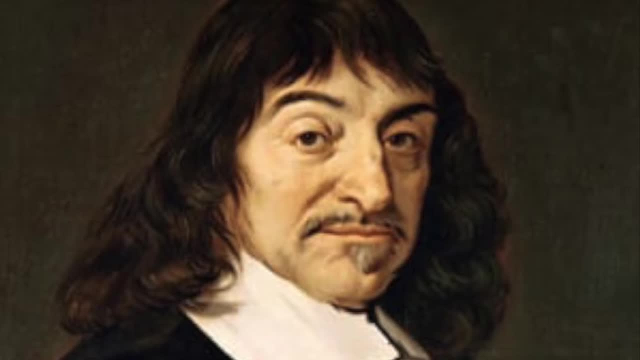 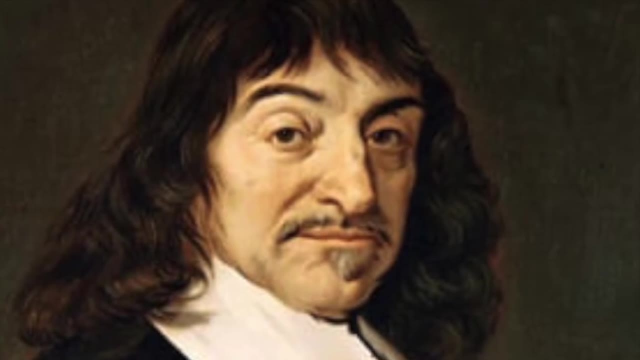 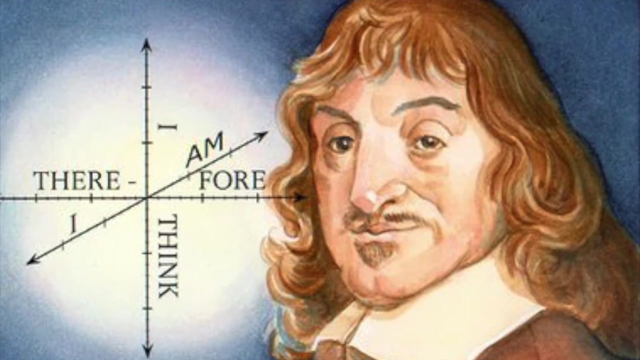 influence on Aristotle and Archimedes. The most notable people who he influenced were all of Western philosophy, but most notably he influenced Sir Isaac Newton and caused the invention of calculus. Aside from the theorem that we'll talk about today, his theorem of circles, Descartes also had one of the most important contributions to math, and 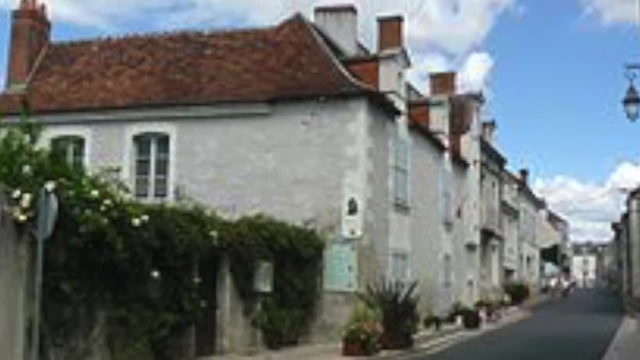 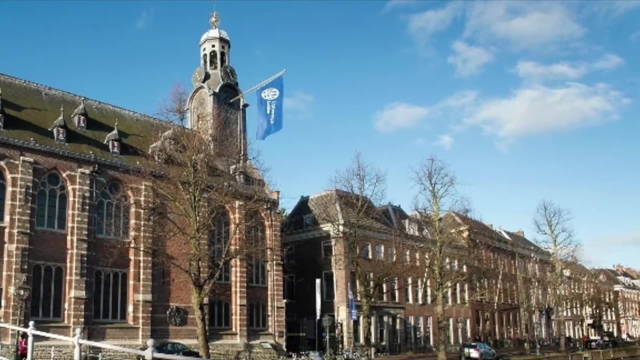 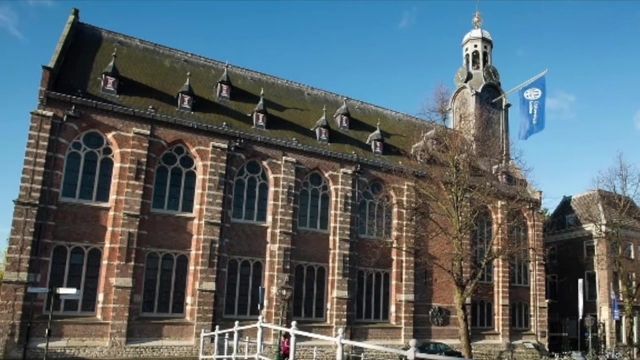 that is, analytical geometry or the Cartesian plane. He made the revolutionary discovery that he could solve problems in geometry by converting them into problems in algebra. He showed that curves could be represented in terms of x and y on a two-dimensional plane and hence as equations in algebra. The Cartesian coordinate system used was named in his honor. 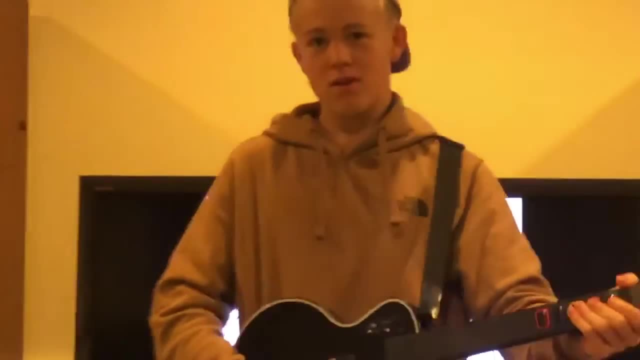 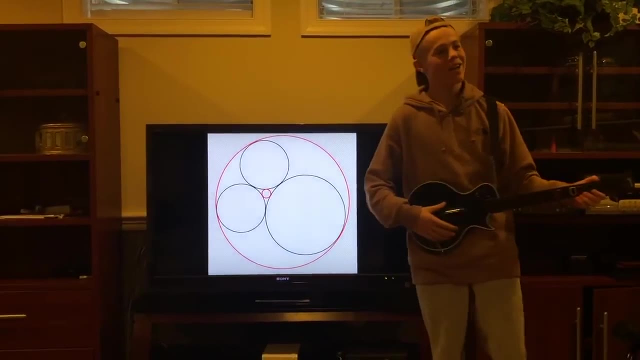 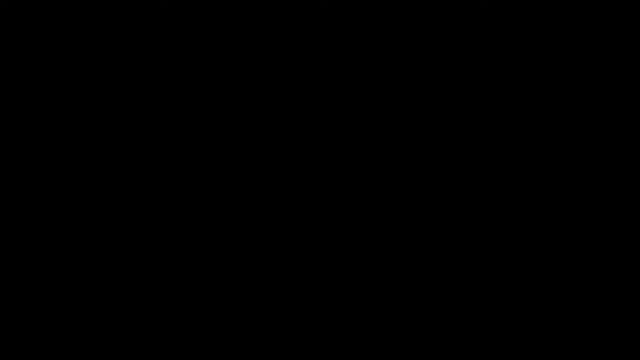 What up, my rock stars. We're back here with another Rockstar, Math, and today we're proving Descartes' theorem of circles. And here, to explain what it is, is my main man, Ronnie McApatra. Alright, ladies and gentlemen, A little switch up from your regularly scheduled programming. 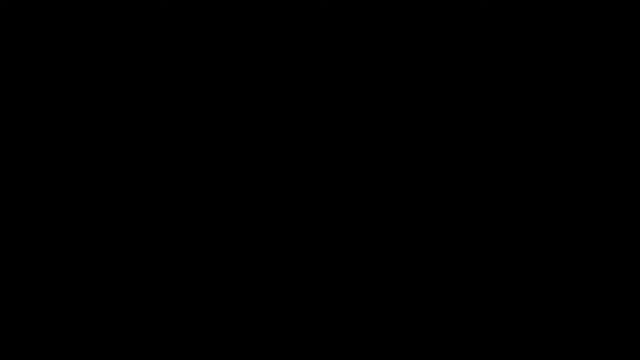 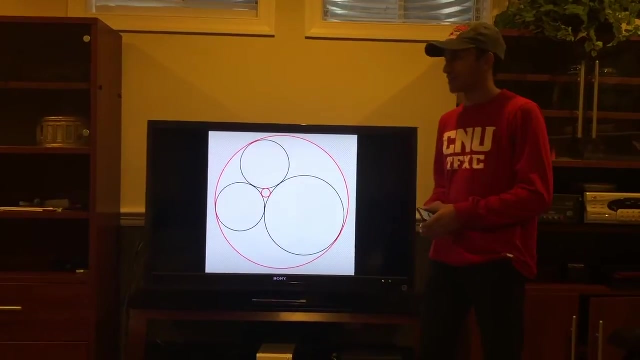 we're taking it back to 1643 for some relaxing Math. We're gonna be joined today by Matt, Ronnie and Luke, who are going to be teaching you all about Descartes' Circle Theorem. Stay tuned for more. Whatup, my rock stars. So basically, Descartes' Circle Theorem proves that there are for. 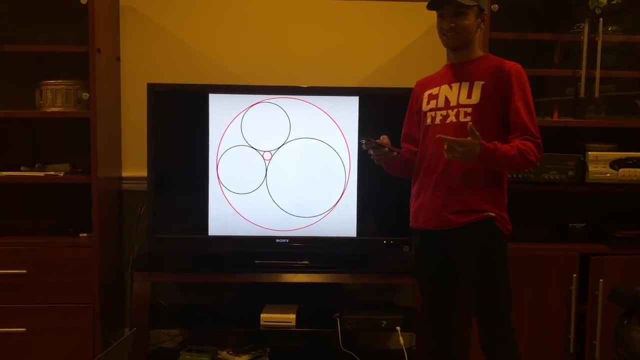 some reason, zero, zero and zero. This is very, very simple. But if we were to turn around and say, hey, why do we have this? It's a very simple thing: for every four kissing mutually tangent circles that there is a quadratic. 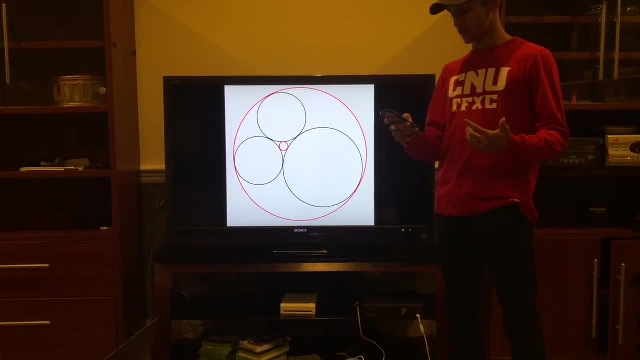 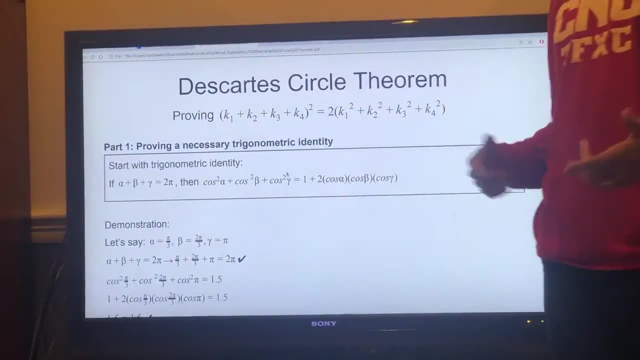 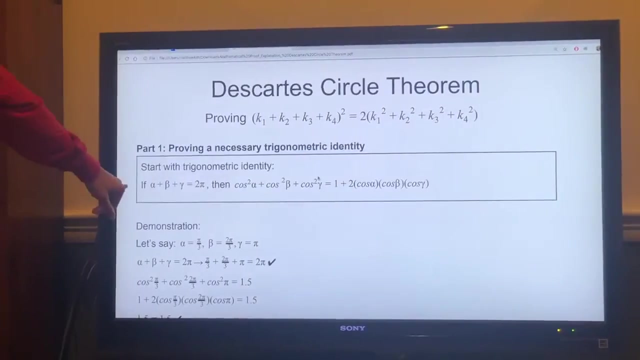 equation that can be solved to find a fourth circle tangent to the three given. So before we start proving the circle theorem itself, we have to prove a necessary trigonometric identity. So basically we start with: if alpha plus beta plus gamma equals 2 pi, then cosine squared of alpha plus cosine squared of 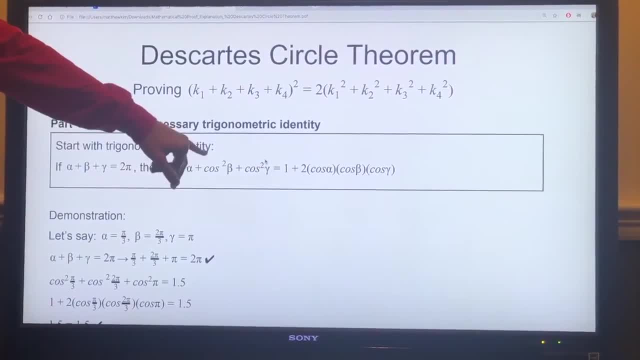 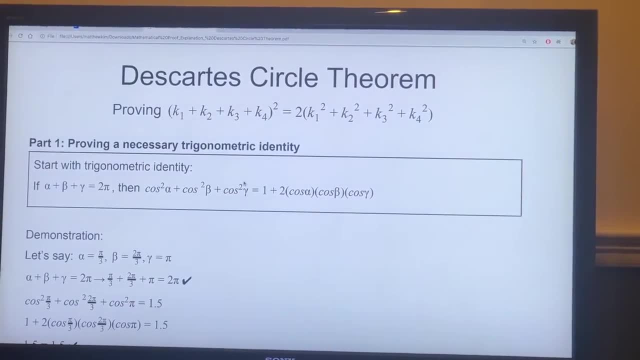 beta plus cosine squared of gamma equals 1 plus 2 times cosine of alpha, times cosine of beta, times cosine of gamma. So to prove it basically, we just plug in three values for alpha, beta, gamma: Alpha equals pi over 3, beta equals 2 pi over 3,. 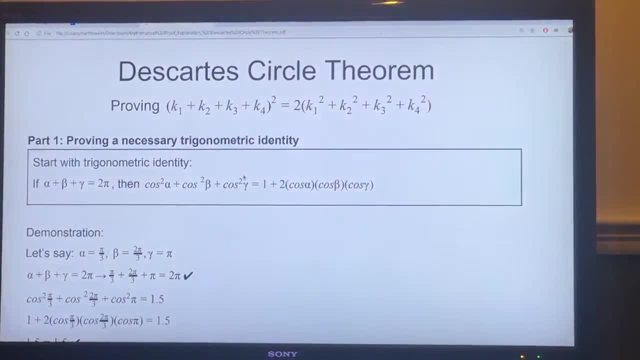 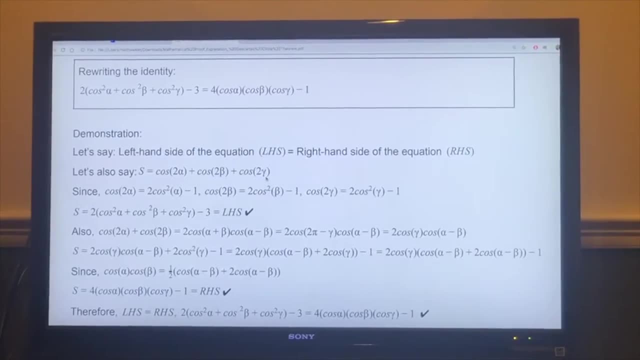 gamma equals pi. Therefore, these three angles equal 2 pi. Then we just plug it in and we just make sure that everything is equal to each other. Step 2 of part 1 is to prove this identity. 2 times 2 pi equals 2 pi. 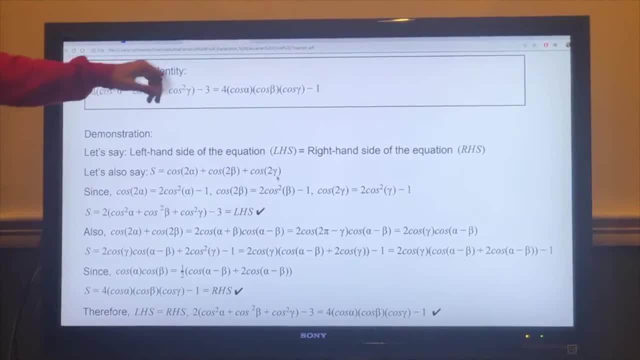 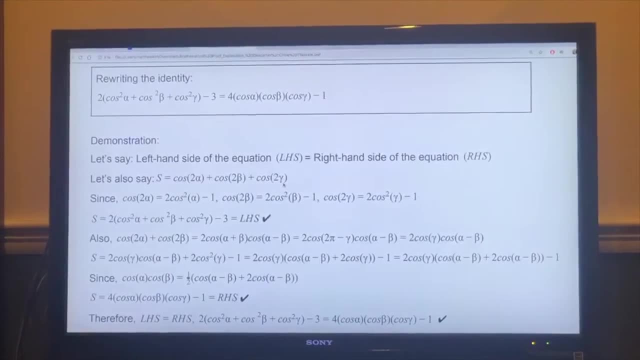 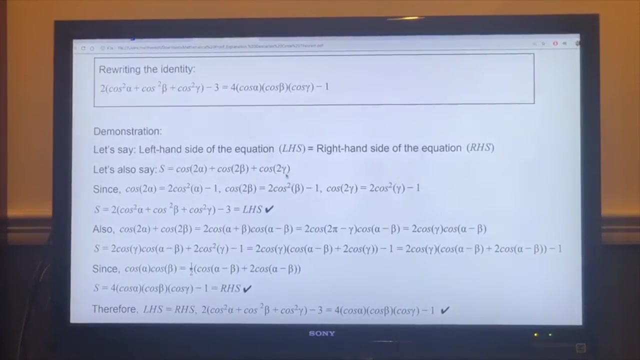 So we'll call this alpha plus cosine squared. alpha plus cosine squared beta plus cosine squared: gamma minus 3 equals 4 times cosine alpha times cosine beta times cosine gamma minus 1.. So what we're going to do here is we're going to split the left and the right and we're going to call this the LHS and the RHS for left hand side and right hand side. 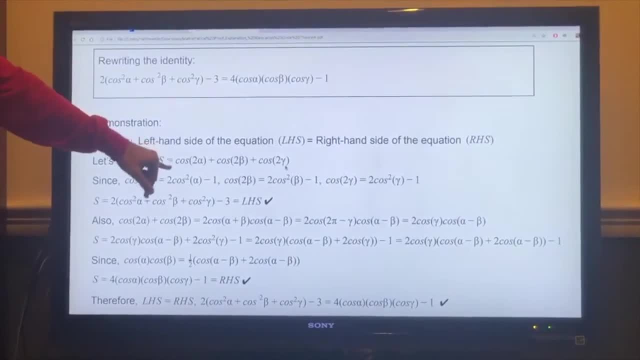 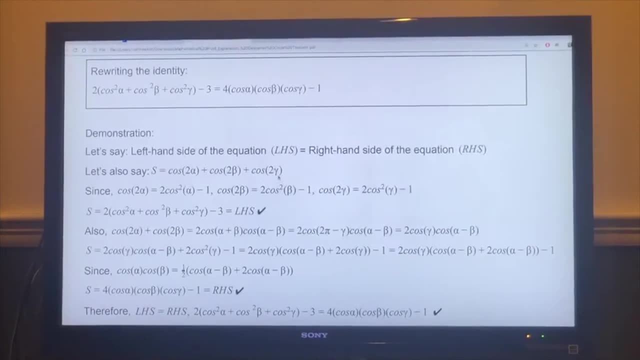 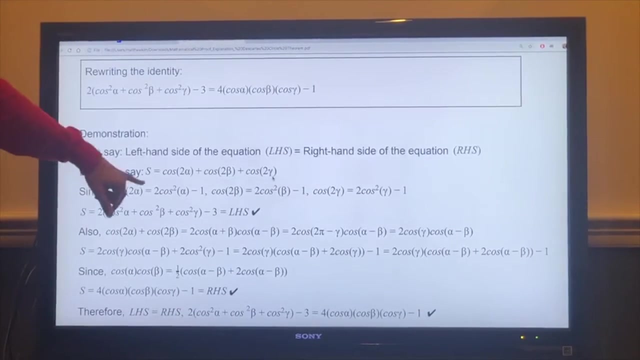 So we're going to start off with S: equals cosine 2 alpha plus cosine 2 beta plus cosine 2 gamma. So, as you recall from precalc, we're gonna remember that the double angle identity cosine of 2 alpha equals 2 cosine squared alpha minus 1.. If we sub in our 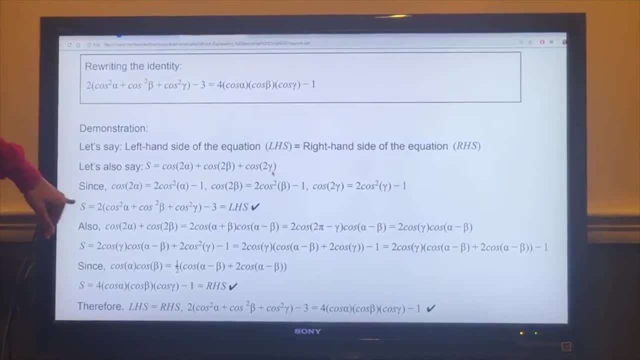 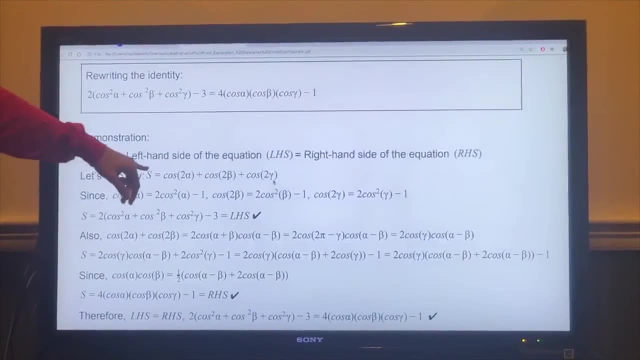 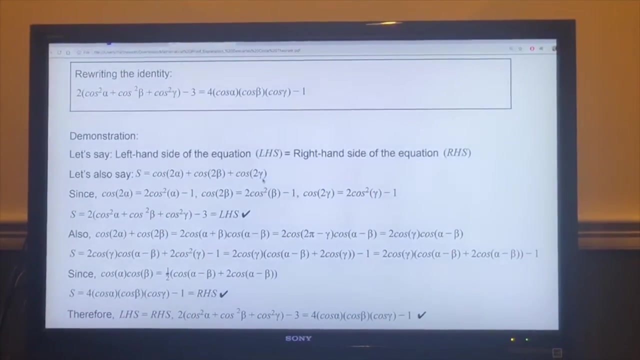 identity into the s equals equation. we ultimately get s equals 2 times cosine squared alpha plus cosine squared b plus cosine squared gamma. minus 3 equals cosine 2 alpha plus cosine 2 beta plus cosine 2 gamma. So now also we can translate cosine 2 alpha plus cosine 2 beta into 2 cosine. 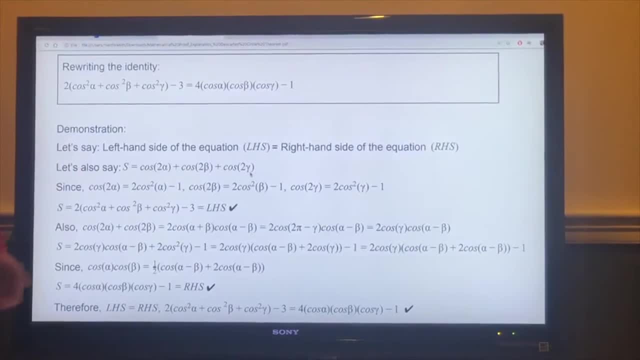 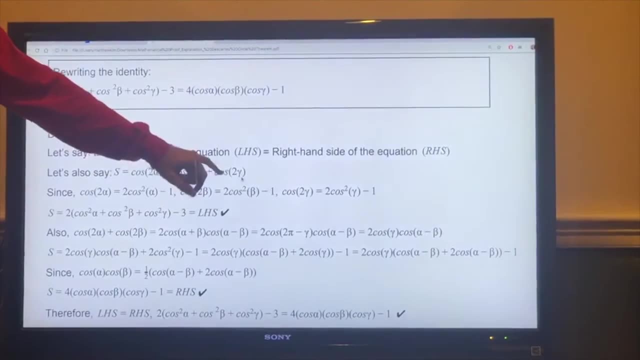 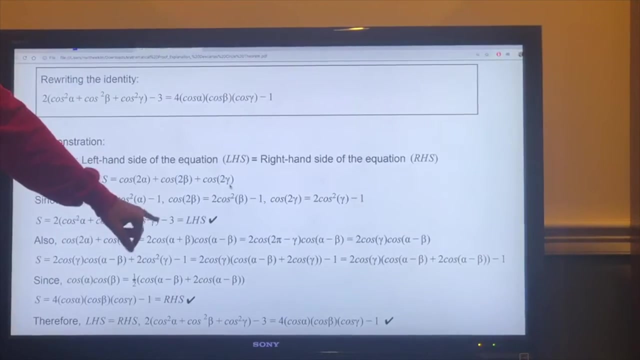 of alpha plus beta times cosine alpha minus beta, which also equals 2 cosine. 2 pi minus gamma times cosine alpha minus beta, which also equals 2 cosine. gamma times cosine of alpha minus beta. We can 2 pi uh 8. alpha plus beta equals 2 pi minus gamma, because alpha plus beta plus gamma. 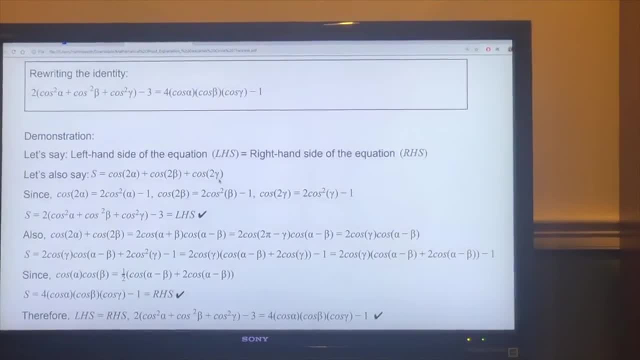 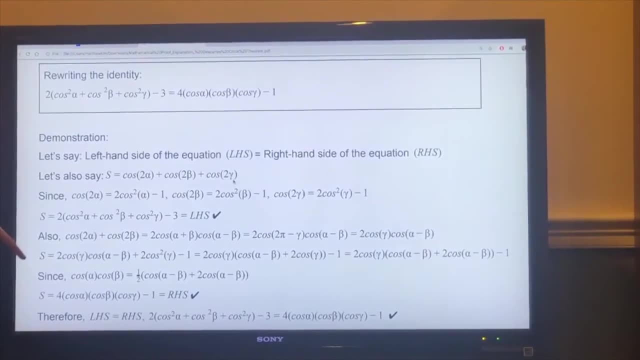 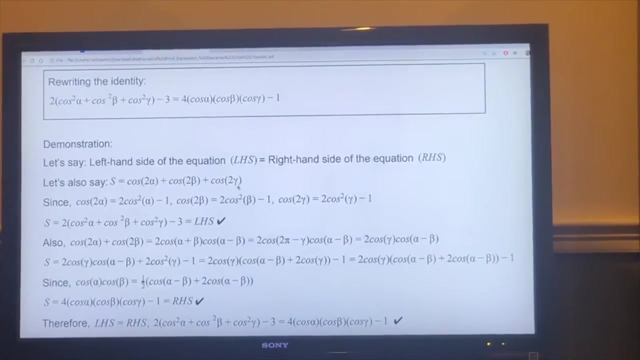 equals 2 pi. So if we keep scrolling down we ultimately get that. s can also equal 4 times times cosine alpha, times cosine beta, times cosine gamma minus 1 equals cosine of 2 alpha plus cosine 2 beta plus cosine 2 gamma. Therefore, the left-hand side equals the right-hand side. 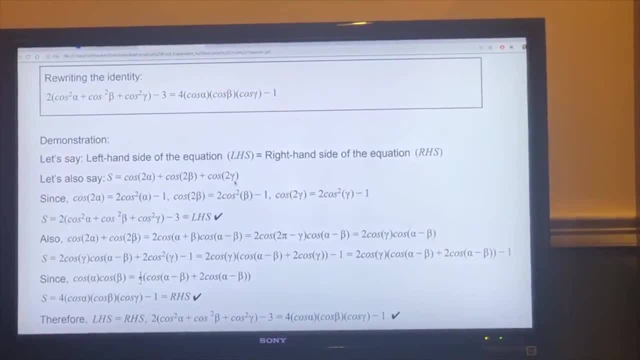 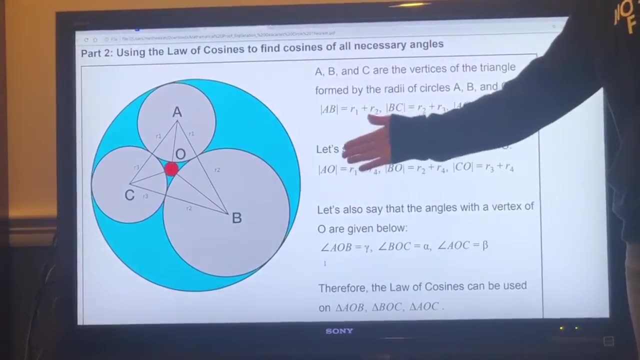 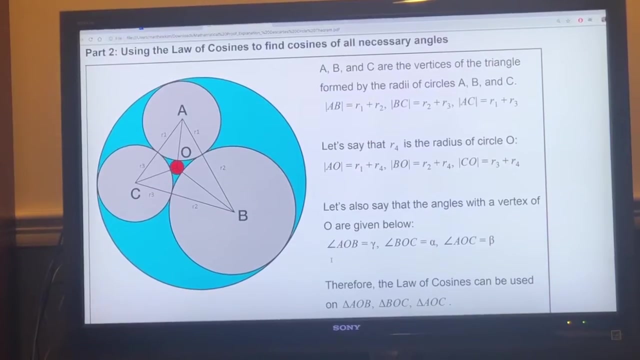 here. So part 2 is using the law of cosines to find cosines of all necessary angles. As you can see, that's the diagram that we previously showed, with the three tangent circles: tangent to a bigger circle, with a smaller circle in between those three circles. If we let 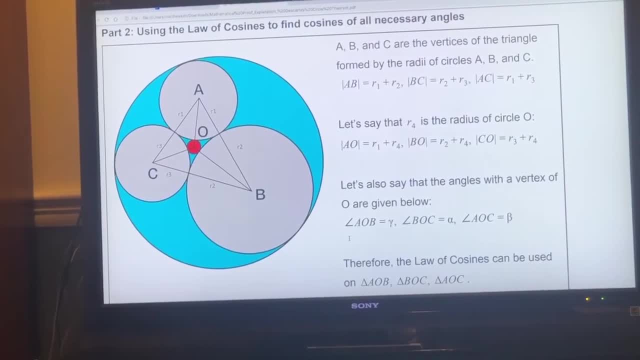 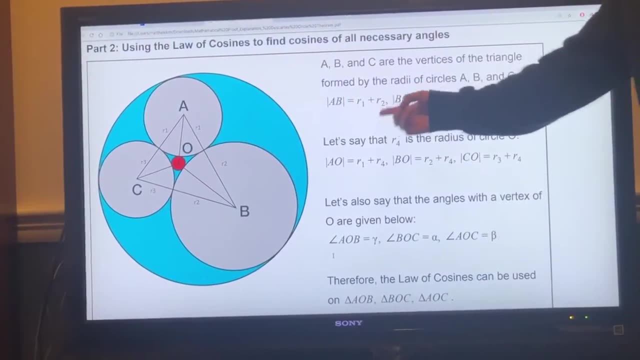 a, b and c be the vertices of the triangle that's formed when we connect the radiuses of the circles. this equation is what occurs. These are the size and that's the different radiuses of the circle. And we also let r4, the radius of the small circle, o, which is 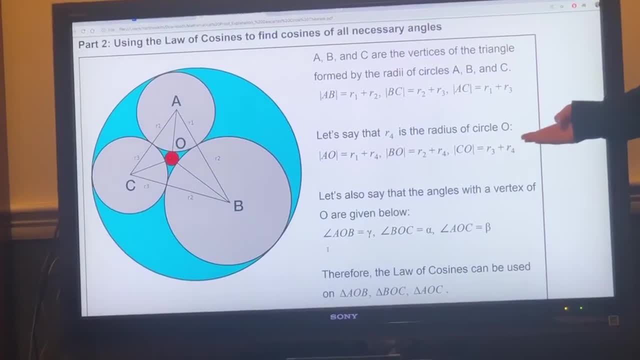 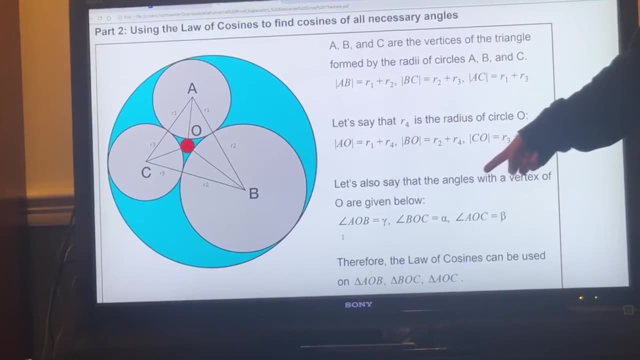 the red circle in the middle, You also get these equations And we also let the different angles of the triangle be the angle a, o, b, b, gamma. So the angle b o c is alpha and angle a o c equals beta. Therefore we can use the 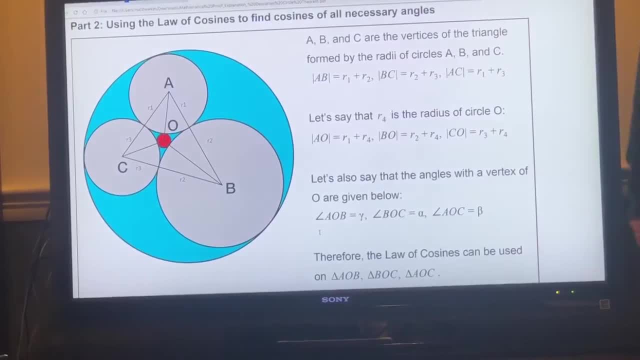 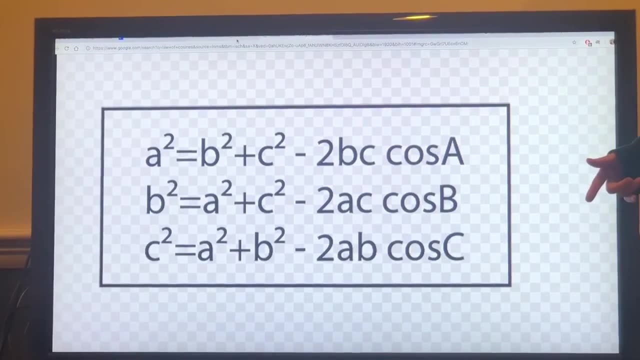 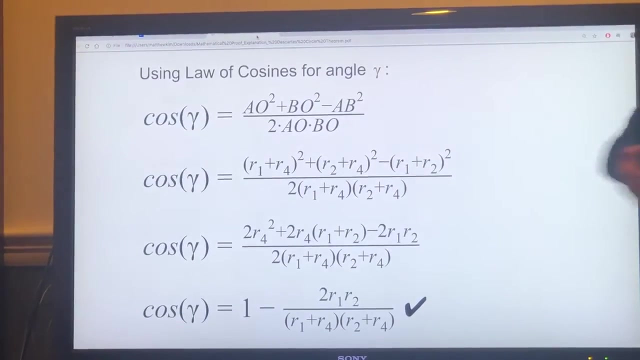 law of cosines on the different angles of the triangle. Just to recall, this is a simplified version of the law of cosines And if we go back to the Descartes theorem, it's the same thing. It's just that instead of a, b and c, a and o, b and o and a, b are just lines. 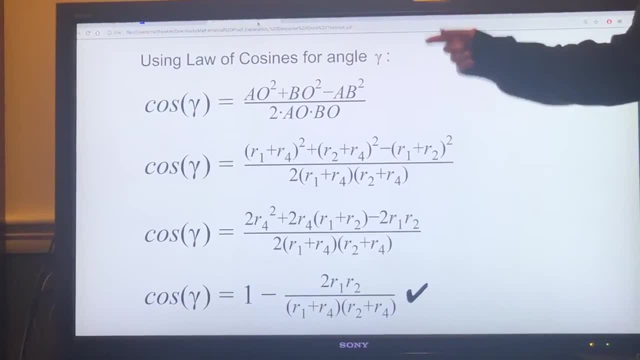 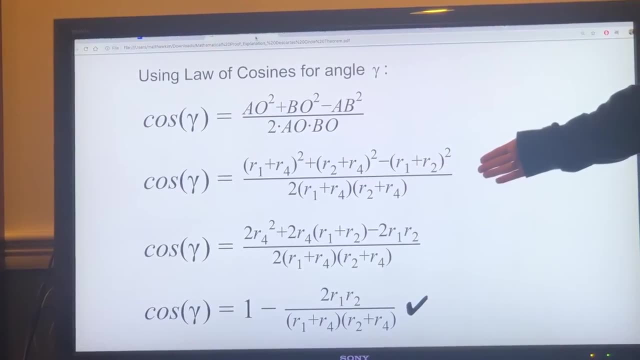 So if we do the law of cosines for angle gamma, this is what occurs. And if you just simplify by simply plugging in the different radiuses that make up each line, you get this equation. And then, just adding everything together, you get this equation and finally, this equation. 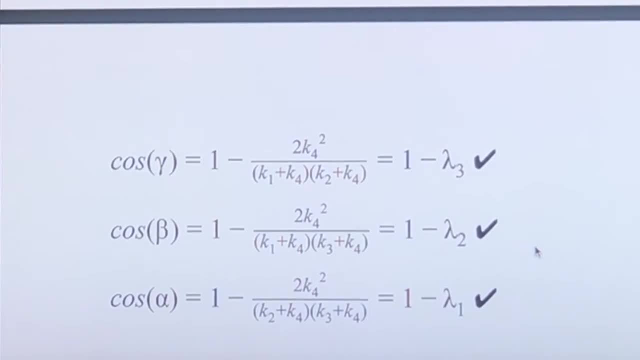 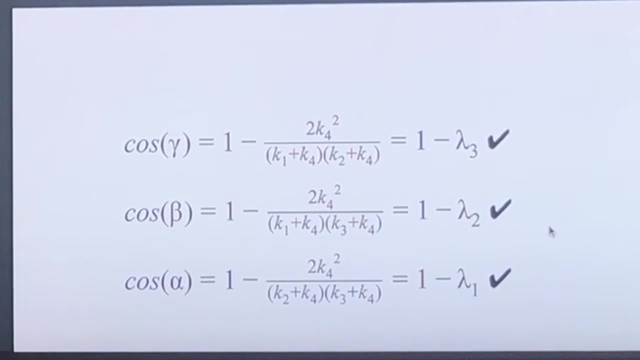 on the bottom. So next we simply use the formula for curvature, which is k equals 1 over r, and replace all the radius variables, so r1,, r2,, r3, and r4, in the equation, And what we get is this equation: 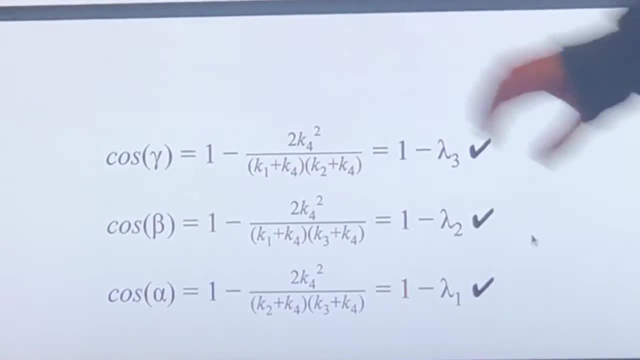 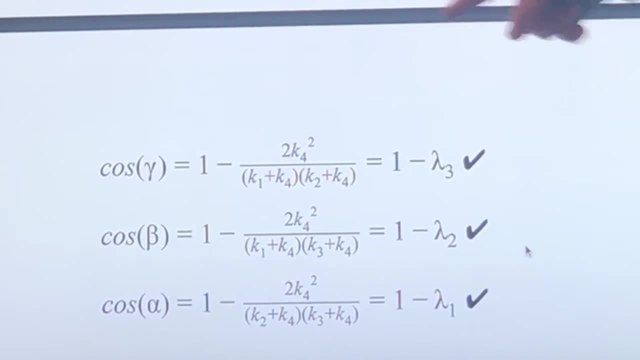 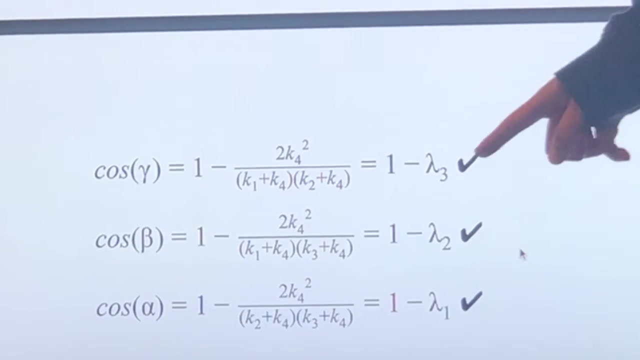 right here, And all we do is simply set this big fraction into different lambdas, since they're all pretty similar, to get a simplified version of: cosine of gamma is 1 minus lambda subscript 3, cosine of beta is 1 minus lambda subscript 2, and cosine of alpha is 1 minus lambda subscript. 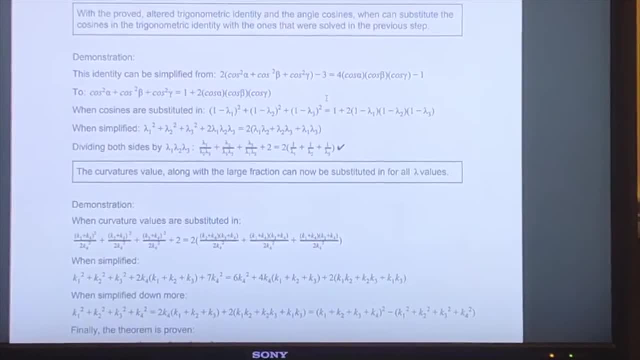 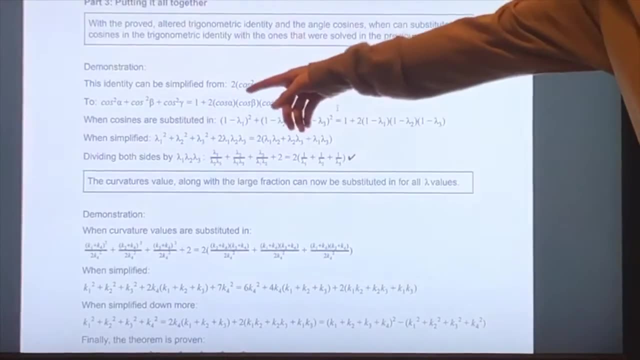 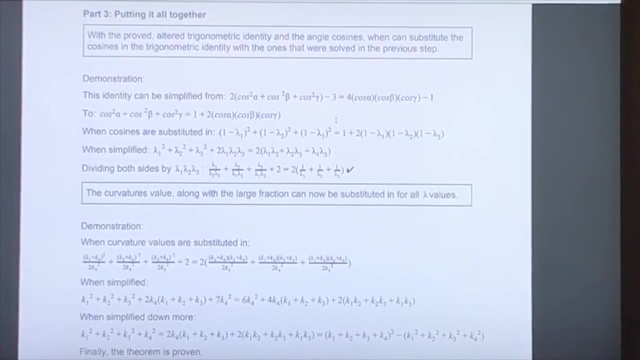 1. Okay, so the last step is just putting together all the information that we got from parts 1 and 2.. So in part 1, we proved that this equation is equal to this one, And so then we're going to use this second equation and we're going to plug in the cosines. 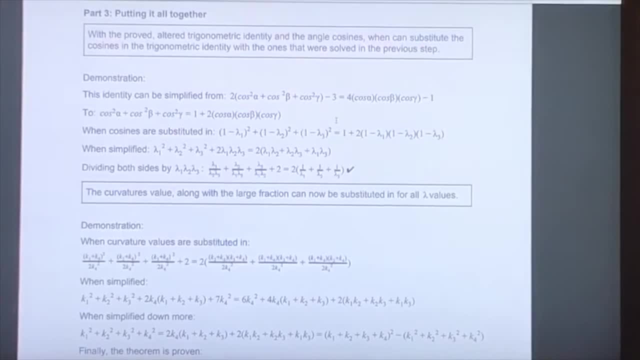 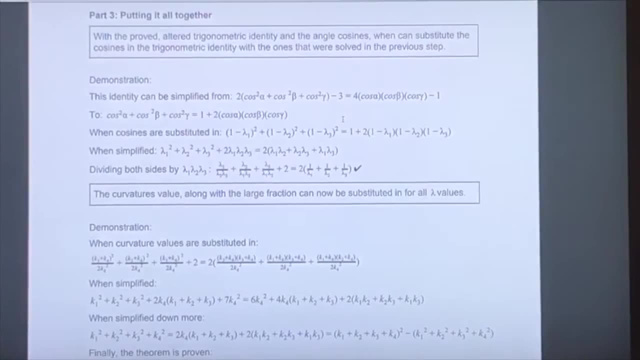 that we got from part 2.. And we get the equation 1 minus lambda subscript, 1 squared plus 1 minus lambda subscript, 2 squared plus 1 minus lambda subscript, 3 squared equals 1 plus 2 times 1 minus lambda times. 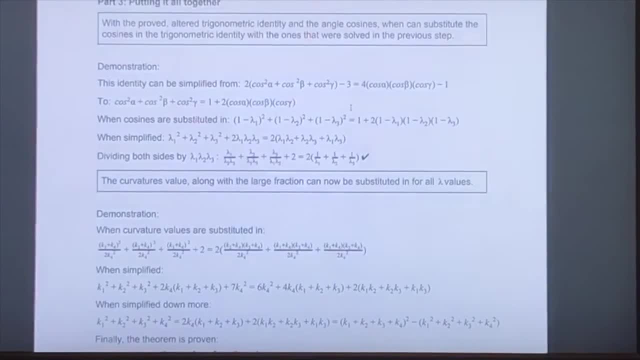 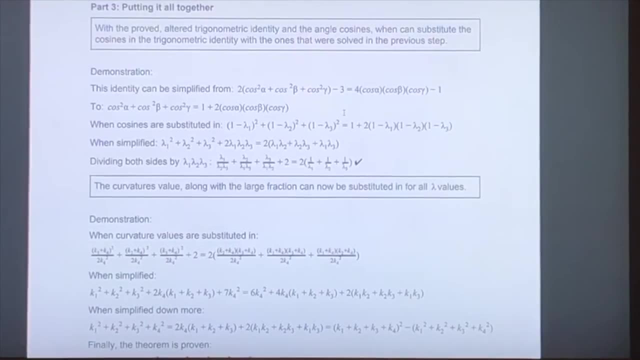 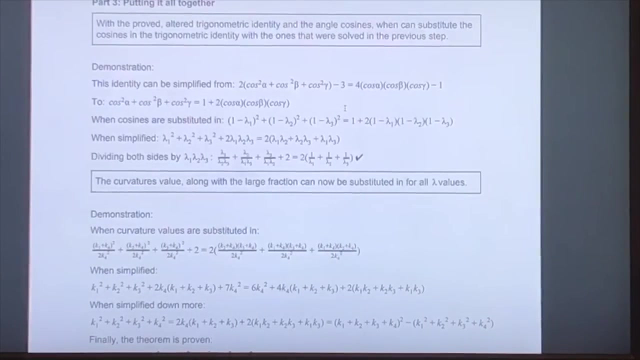 1 minus lambda 2 times 1 minus lambda 3.. So, once simplified, you get this equation right here. And both sides, by lambda 1 times lambda, 2 times lambda 3, we get this equation right here. So, ultimately, the curvature's value, along with the large fraction that we got in part. 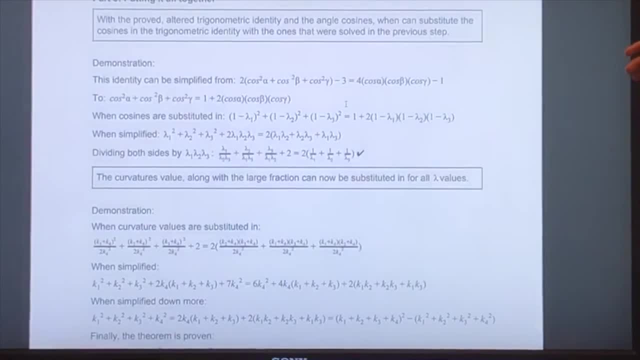 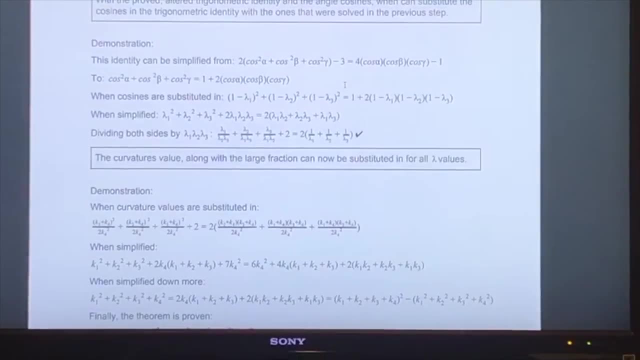 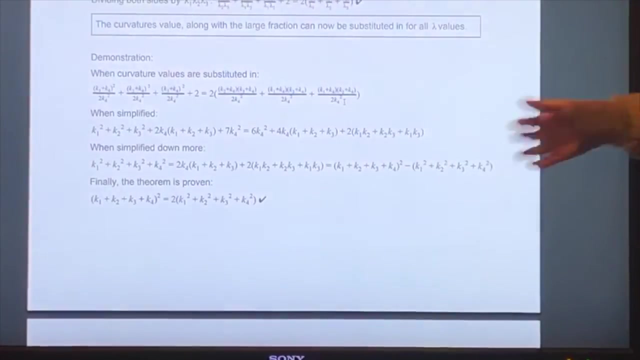 2, can now be substituted in for all the lambda values. So when we substitute them in we get this rather complicated equation, But ultimately when we simplify it down, we get here and continuously simplifying it so that we get a more easy to look at equation. 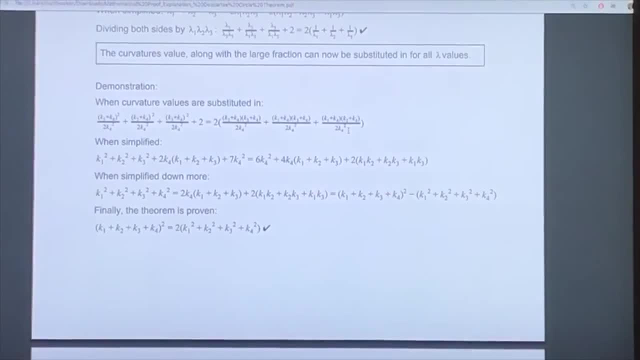 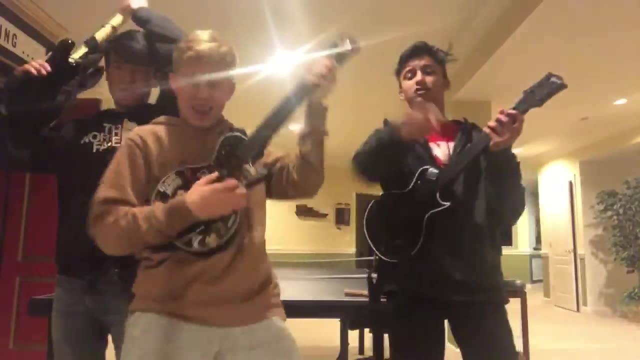 We get the final theorem that we've been trying to get all along and the theorem's completed. Thank you for watching. We hope you learned a lot about Descartes. Subscribe to our YouTube channel. Oh shit, Subtitles by the Amaraorg community.